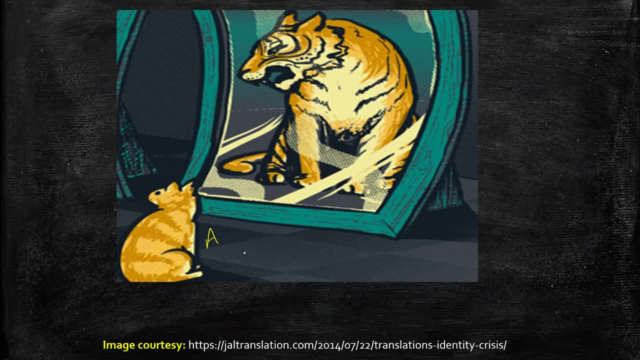 this picture, this cat, is the non-empty set A called the domain. This frame of the mirror is the target set for set B and this image is the transformation of this cat and is called the image set. Now let us move on to the definition of. 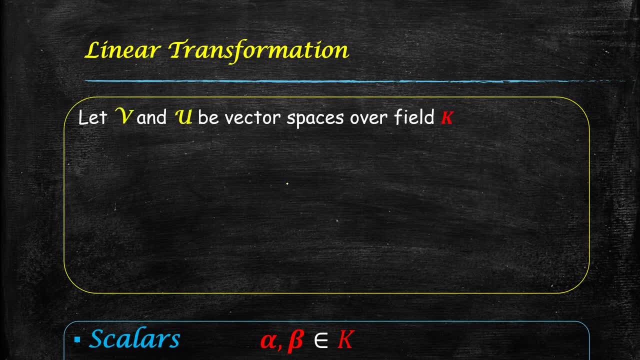 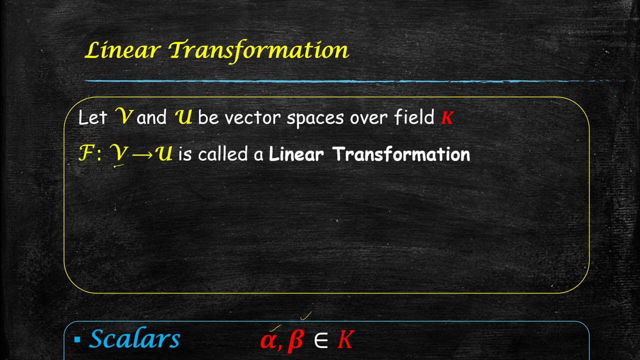 linear transformation. Let U and V be vector spaces over a field K, where K will be either a real or complex number in this lecture, and alpha, beta are the scalars belonging to that field V. Now any mapping F from V to U is called a. 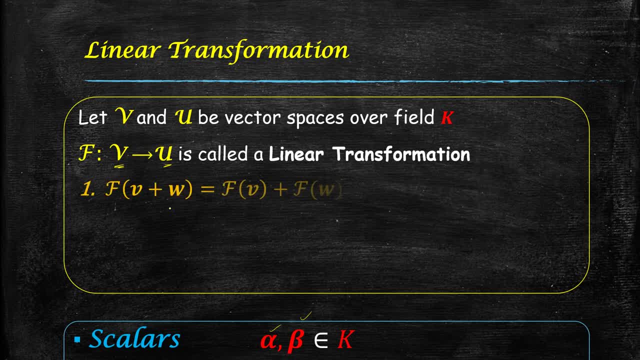 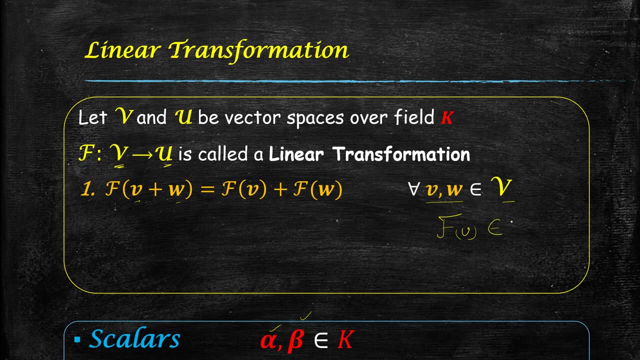 linear transformation if it preserves vector addition, that is, F of V plus W equals to F of V plus F of W. Here V and W are the elements of vector space V. Now F of V and F of W are the elements of vector space U. By this condition. 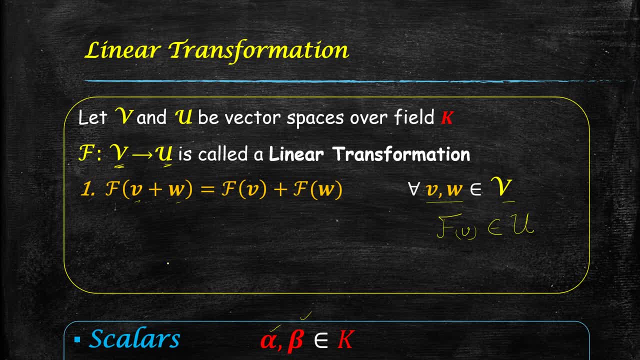 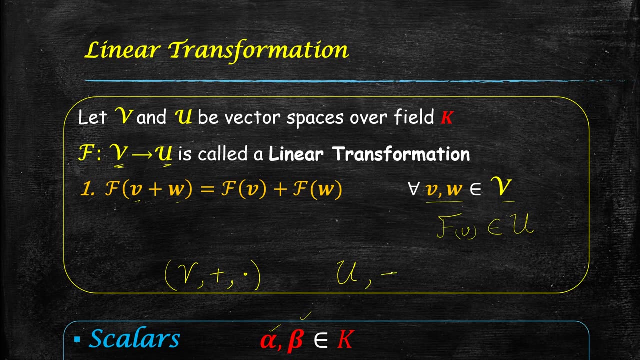 transformation preserves vector addition. we mean here that if V is the vector space together with the binary composition, plus and scalar multiplication, dot, and U is the vector space, with binary composition, vector addition marked as plus, circ and scalar multiplication mark as dot, circ. Now, vector addition of vector space, U and. 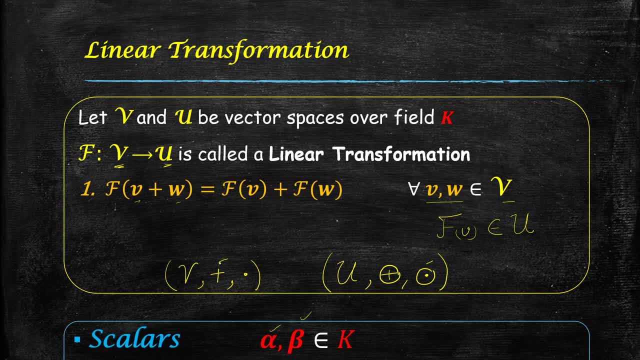 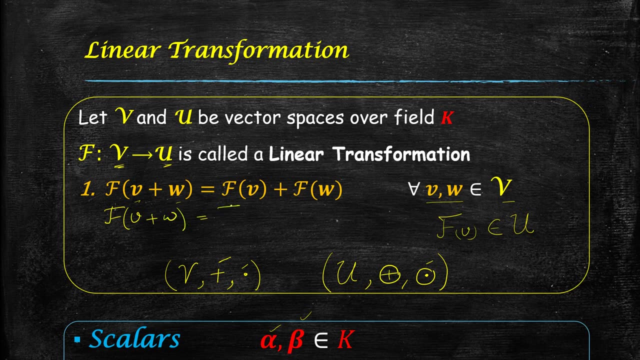 scalar multiplication of vector space U, different from the vector space U, and scalar multiplication of vector space V. So F of V plus vector addition of vector space V and scalar multiplication of the vector space V. By preserving the vector addition here, we means that F of V plus W is equal to. 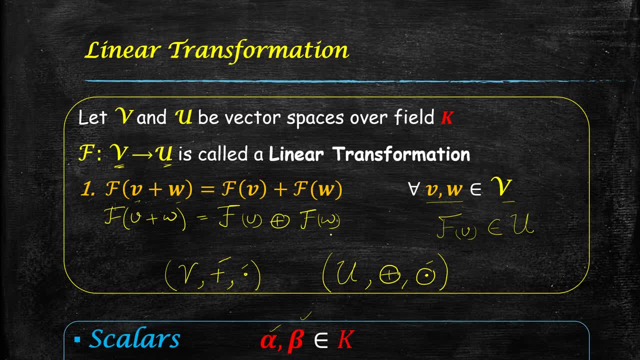 F of V circ plus F of W, because F of V and F of W are the elements of U. Therefore the vector addition will be from the vector space U. F of V to U is called a linear transform of vector space U if it preserves vector addition number one, number two, if it preserves scalar. 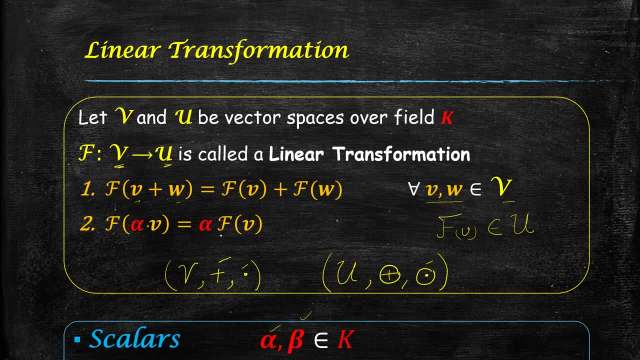 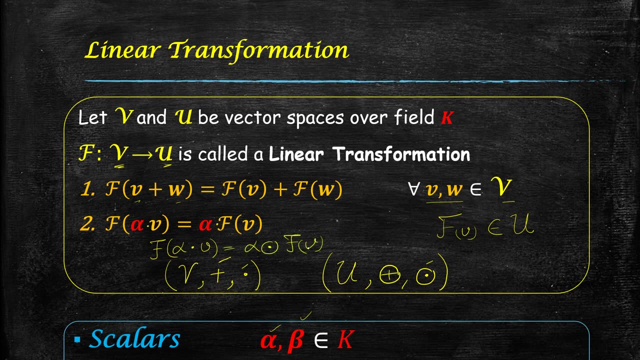 multiplication F of alpha into V is equal to alpha F. preservance of scalar multiplication is same as the previous. we can say here that F of alpha into V is equal to alpha circ F of V. for simplification, throughout the lecture we will consider that vector addition and scalar multiplication, for both the 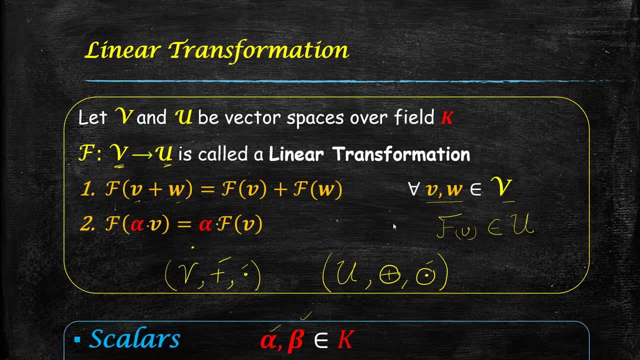 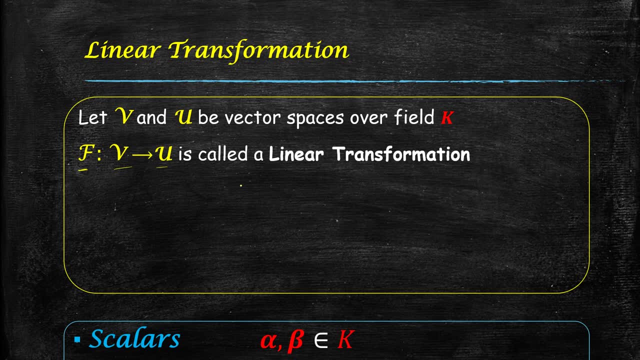 vector spaces will be same. more generally, if I combine these two conditions, I can say that a mapping F from V to U is called a linear transformation, if, and only if, F of alpha, V plus beta W, where alpha, beta are scalars, equals to alpha into F V plus beta into F W. our second definition is about linear operators. now 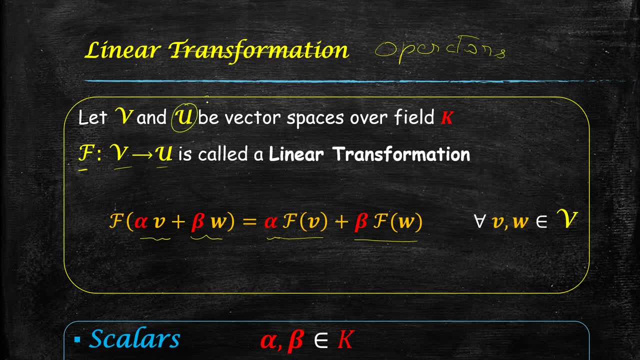 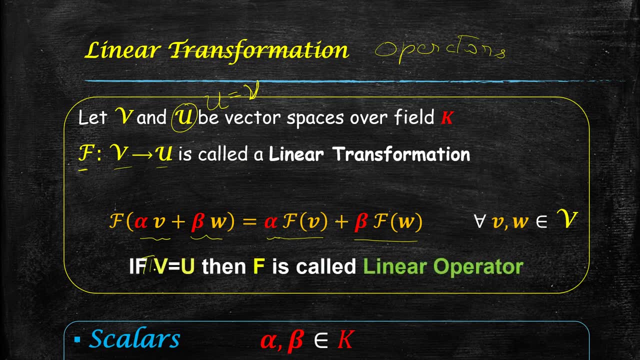 in this definition, if vector space U is equals to the vector space of the vector space of the vector space of the vector space V, what I am saying? that if U and V both have the same vector space, then we say that linear transformation is linear operator. the examples of linear 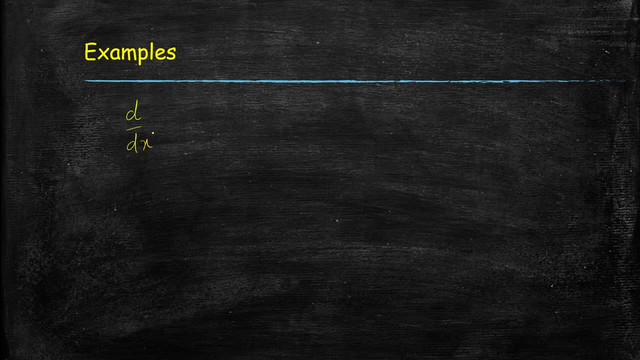 operators are D by DX is the differential operator, integral operator, because in both transformation the domain and range will be. so I will write vector space mean as V by linear operator as f from vector space V to. we know up to top is linear operator as add from vector space V to vector space. 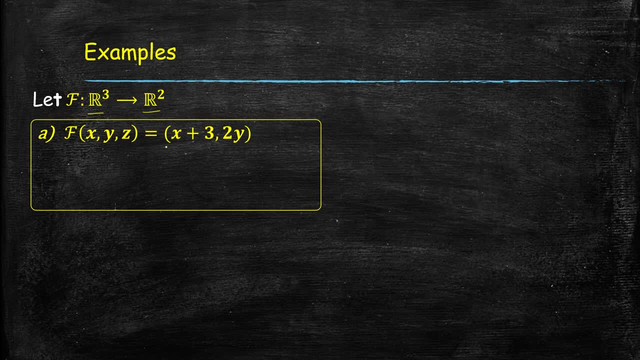 let us discuss some examples. let fp, a transformation from vector space, are string to our sphere. our first example is f of X, YZ equals to X plus 3 to y. the question is rather: this transformation is linear transformation? are not now here? purchase equation now here, if V belongs to our three, then we will be of the type: say x, 1, y, 1. this transformation will be linear. 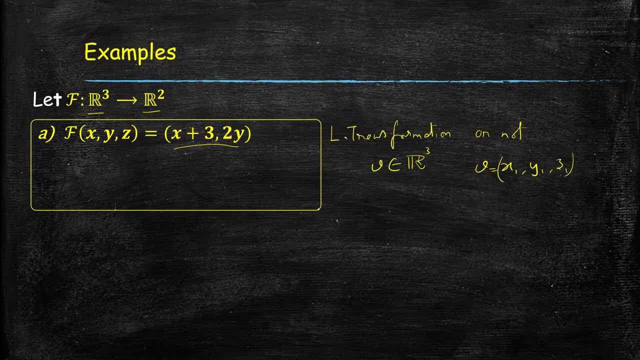 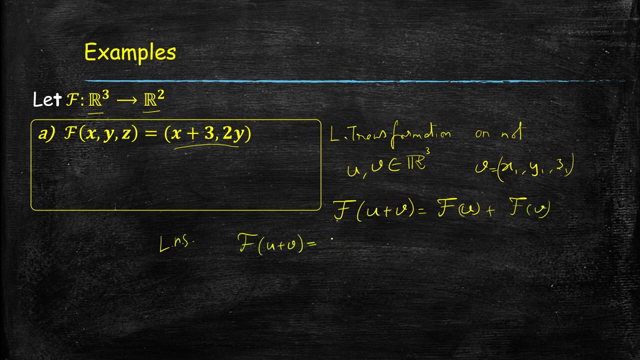 Ans. This transformation will be linear transformation. if for any u and v belonging to R3, f of u plus v is equals to f of u plus f of v. Now the left hand side here is f of u plus v, which is equals to say f of x1, y1, z1 for v plus x2, y2, z, or equivalently x1 plus x2, y1 plus y2, z1 plus z. 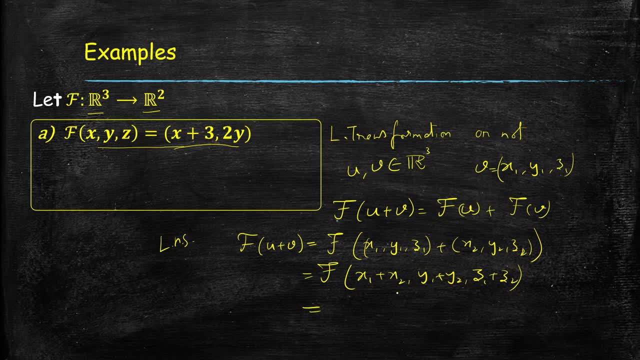 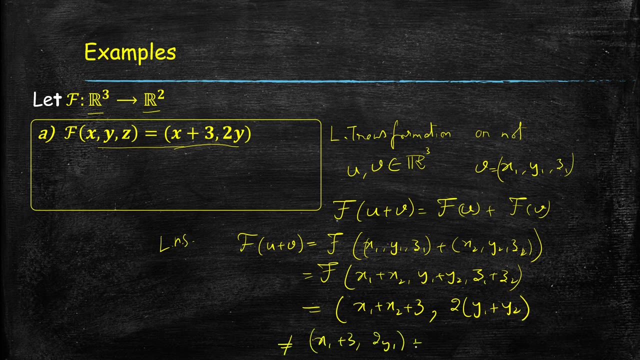 By the definition of linear transformation, f of x1 plus x2, y1 plus y2, z1 plus z2 equals to x1 plus x2 plus 3 comma, 2y1 plus y2.. But this value is not equals to x1 plus 3, 2y1 plus x2 plus 3, 2y, which is f of u plus f of. 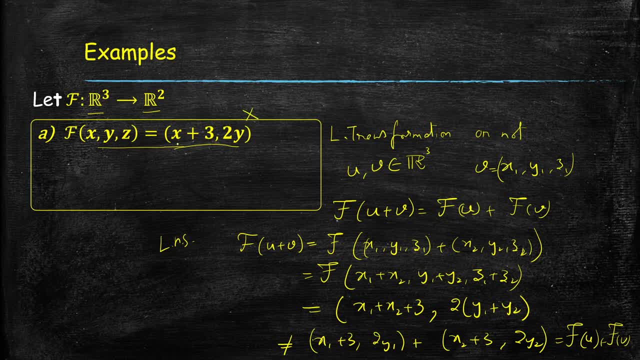 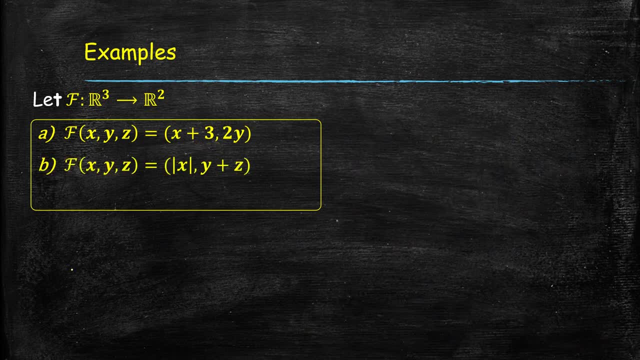 So this transformation is not linear transformation as it does not preserve vector addition. Let us move on to second example: mod x, y plus z. Mod x1 plus x2 need not to be equal to mod x1 plus mod x2.. So in this transformation, if you will try to find out f of v plus w, then it come out to be mod of x1 plus x2, y1 plus y2 plus z1 plus z. 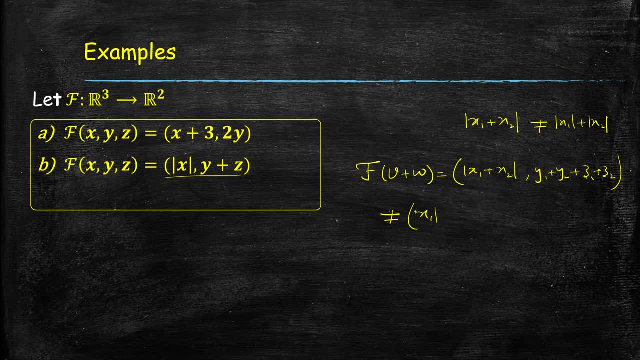 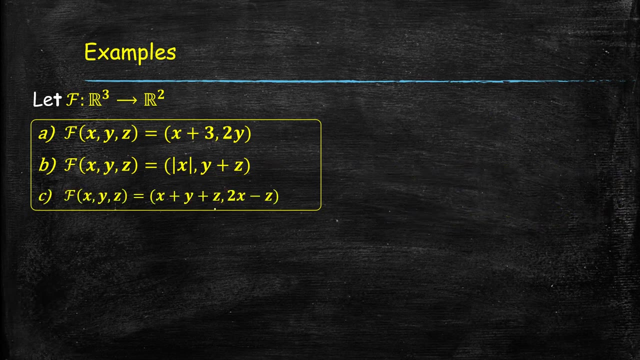 But this is not equal to mod of x1, y1 plus z1 plus mod of x2, y2 plus z2.. So this example is also known. So this is not a linear transformation. Let us try another example: f of x, y, z, x plus y plus z, 2x minus z. 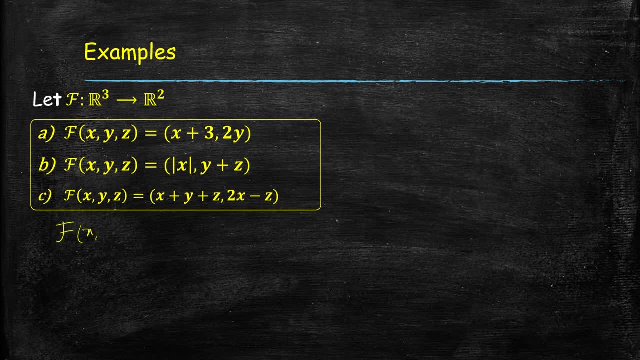 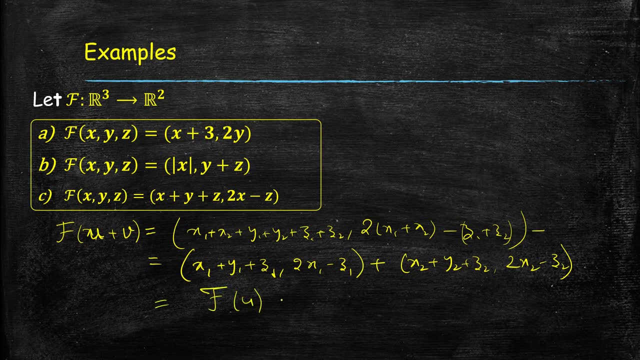 It is easy to see here that this transformation is linear transformation. u plus v equals to. on solving you will get is equals to fu plus fv. Similarly, we can show that f of alpha into v equals to alpha fv. It is an example of linear transformation. 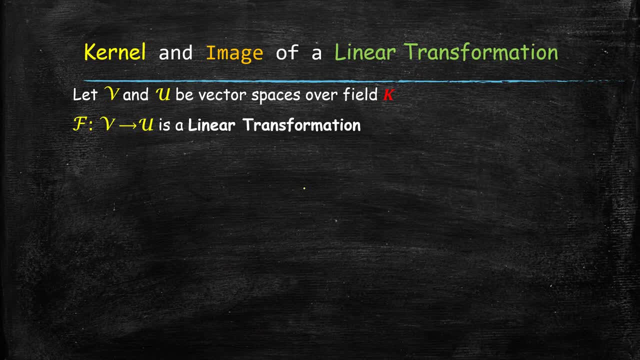 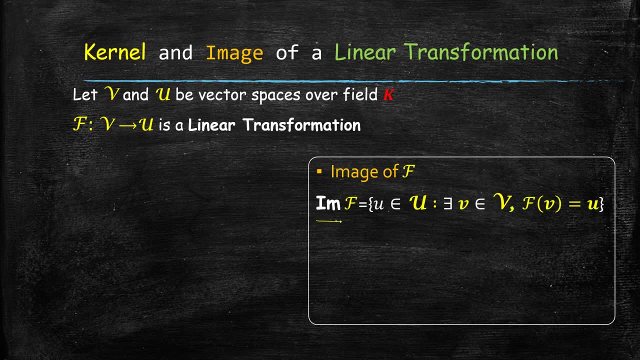 Next definition of kernel and image of a linear transformation. So our first definition here is the image of f, The image of linear transformation. f is defined as those elements of u, such that f of v equals to u for some v belonging to vector space v. 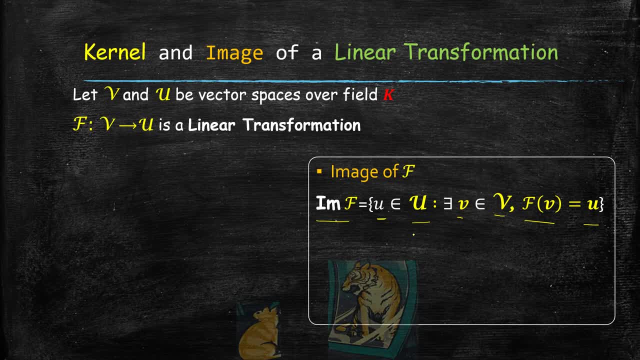 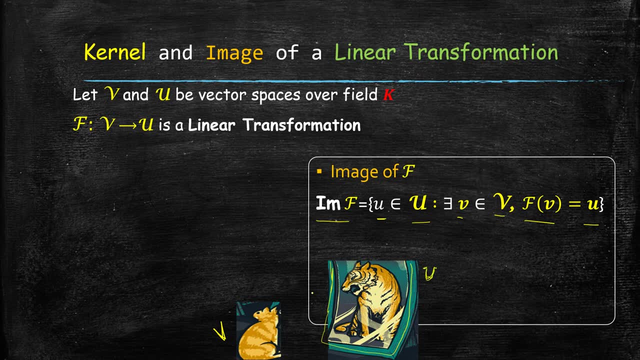 If you could remember our example of cat and tiger Here, assume that this cat is the vector space v And this mirror is the vector space v. The image of f here is our tiger. This tiger is transformation of this cat. Image of f are those elements of vector space u such that u equals to f of v for some v in vector space v. 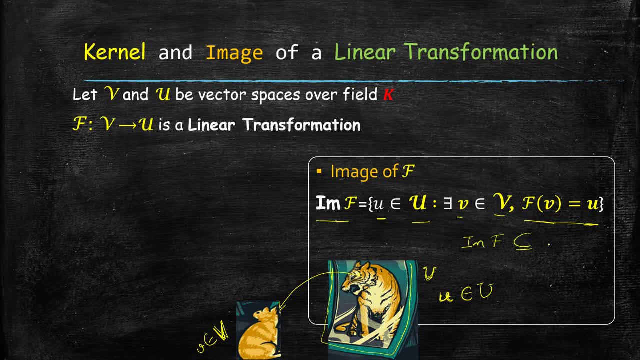 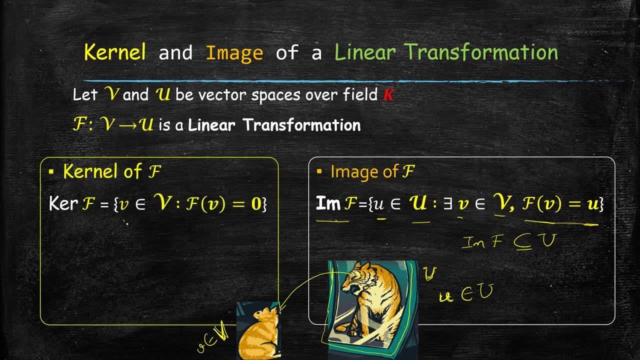 Here you can see that image of f is subset of vector space u. Our next definition is about the kernel. Kernel of f is defined as Those elements of vector space v. Image of v is zero vector Kernel of f: here is subset of vector space v. 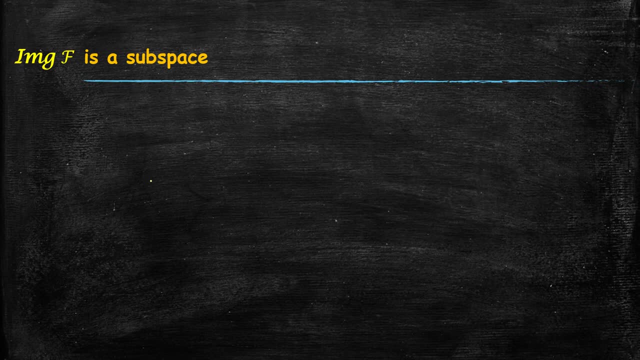 Next, we will prove that image of f is a subspace, As we all know that any subset w of a vector space, v, is called a subspace if, and only if, w is itself a vector space. And to prove that w is a vector, 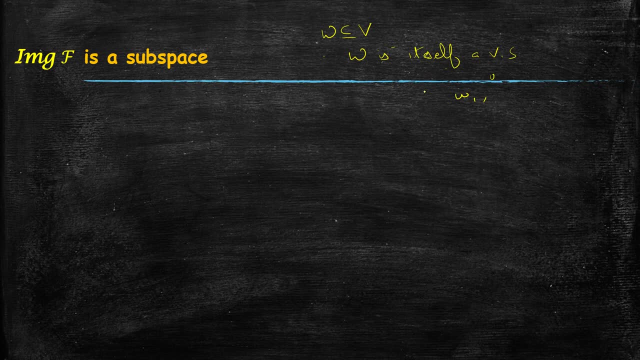 We have only to show that For every w1, w2 belonging to w, Alpha of w1 plus beta of w2 also belongs to w, Where alpha beta are scalars from the field f. So here, if I want to prove that image of f is a subspace, 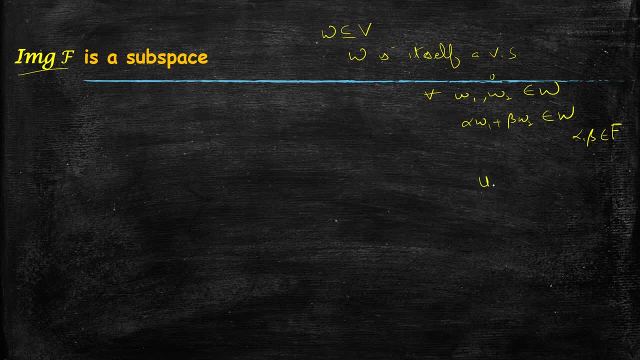 I only need to show that if u1 and u2 are elements Of image of f, Then alpha u1 plus beta u2 is also an element of image of f. If I could prove that, then I can show that image of f is a subspace. 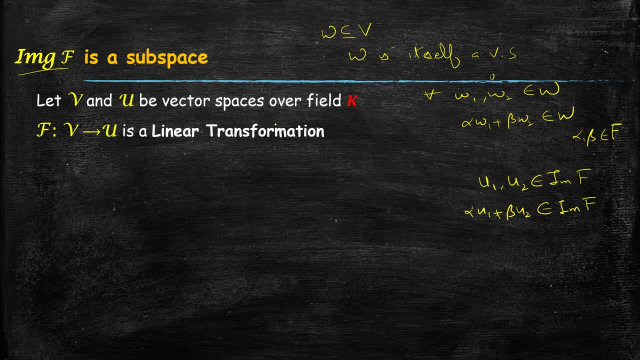 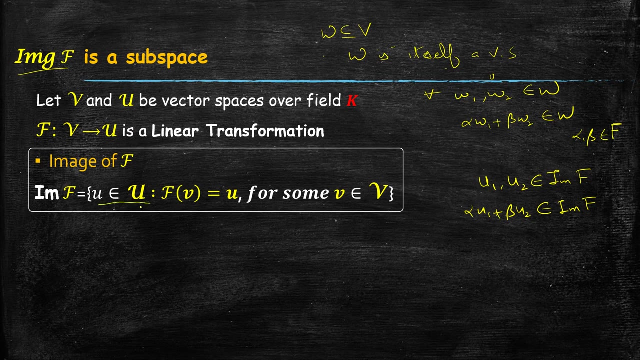 Let us start with some basic notation. Let v and u be the vector spaces over a field k. F be a linear transformation from vector space v to u, And you all know that image of f is defined as Those Elements of vector space u, such that fv equals to u. 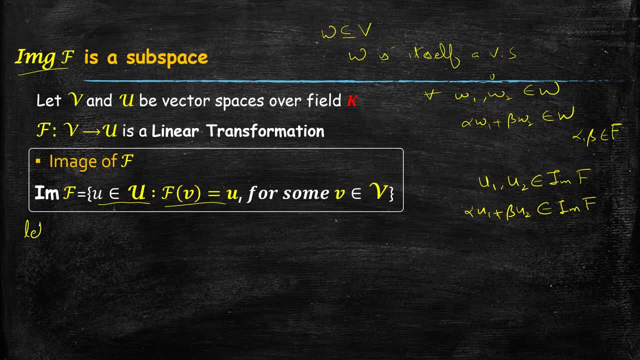 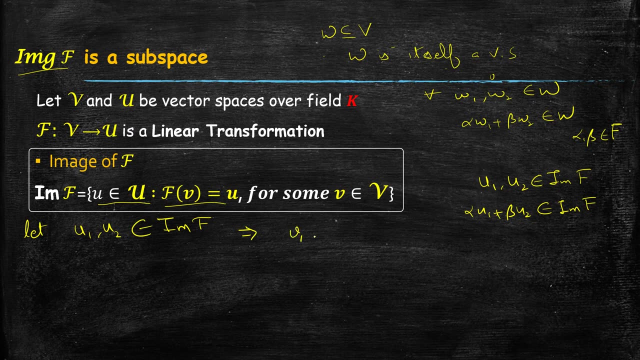 For some v in vector space v. Now, if assume that u1 and u2 belongs to image of f, Now u1, u2 belongs to image of f implies that there exists some v1 and v2 in vector space v, Such that f of v1 equals to. 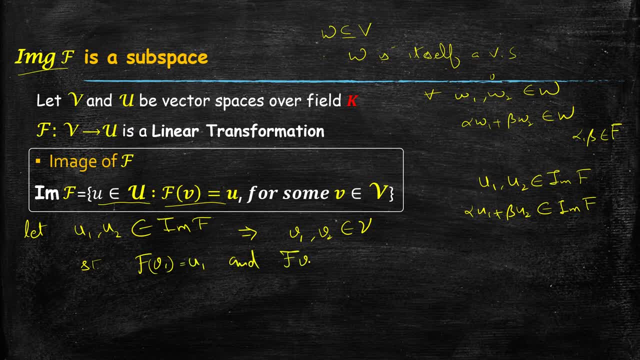 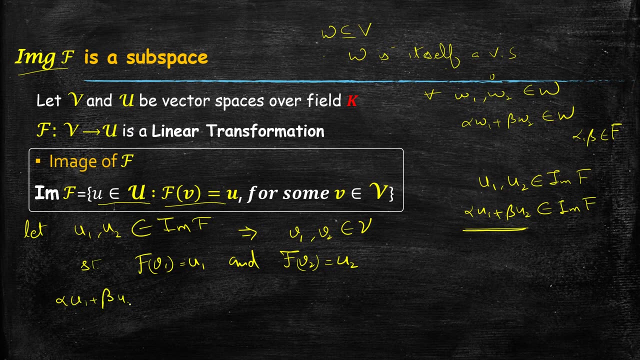 u1 and f of v2 equals to u2.. And I will show that alpha u1 plus beta u2 also belongs to image of f. So let us start with alpha u1 plus beta u2.. Now u1 equals to f of v1. 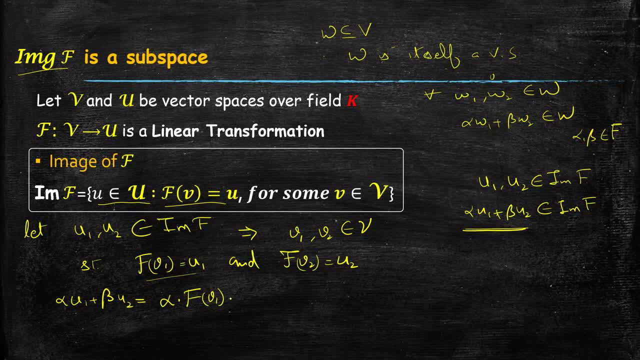 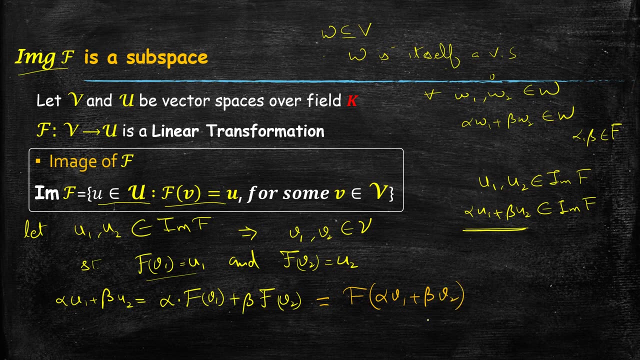 So I will write here alpha f of v1 plus beta f of v2.. But f is A linear transformation. Therefore this is equals to f of alpha v1 plus beta v2.. By definition of linear transformation. So I can say here that for alpha u1 plus beta u2.. 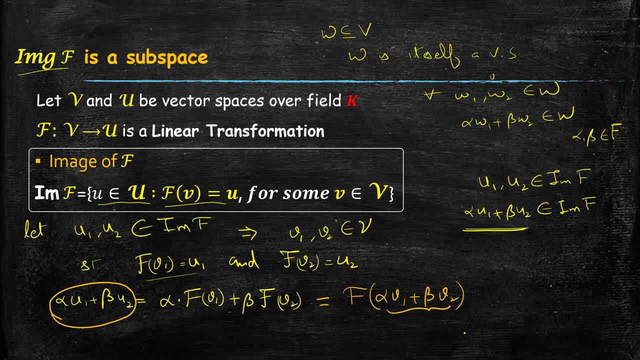 There exists some element of vector space v, Such that f of those element of v equals to alpha u1 plus beta u2.. But that is the definition of image Of f, which says that image of f contain those elements u, Such that there exists some element of vector space v. 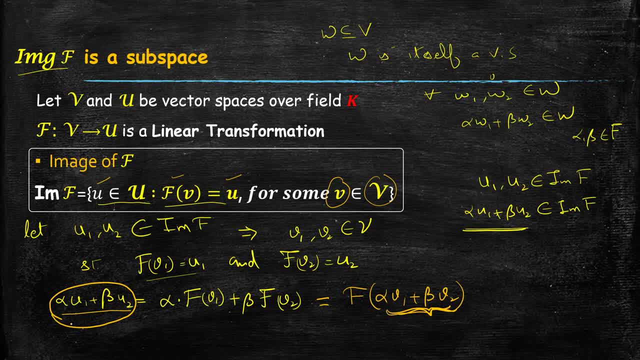 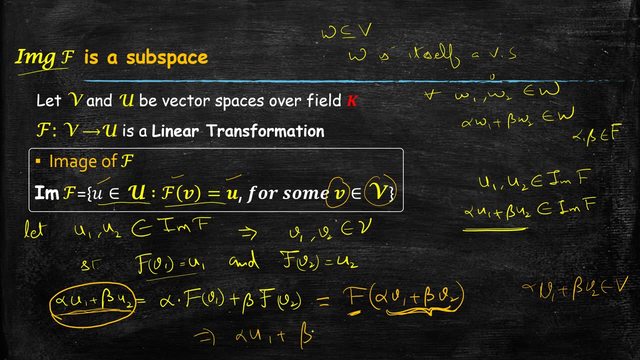 For which f of v equals to u. And here I am also saying that there exists some element of v Such that alpha u1 plus beta u2 is image of that element of v. This means alpha u1 plus beta u2.. Belongs to: 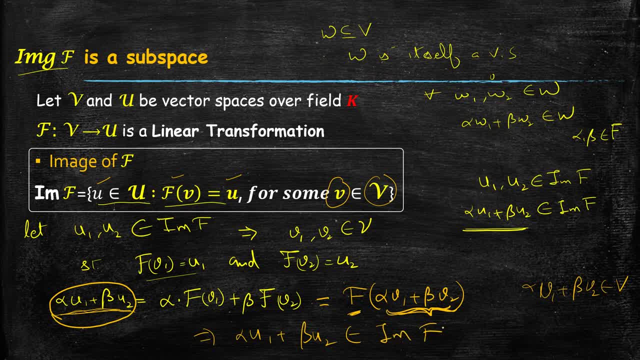 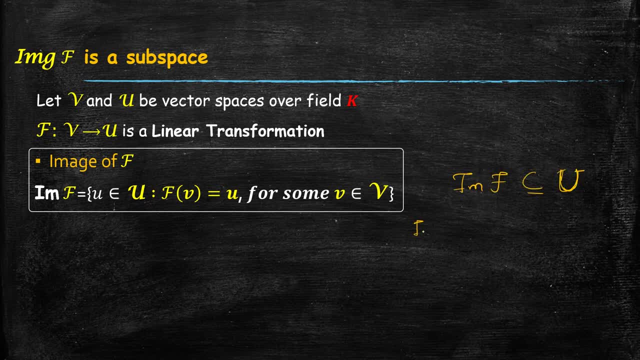 Image of f. Hence, image of f is a subspace. I will repeat this again Now: as image of f is a subspace, Image of f is also a vector space. This means there exists some basis of image of f And there will be dimension of image of f. 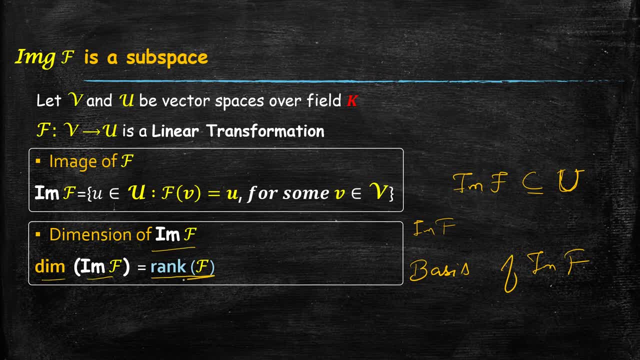 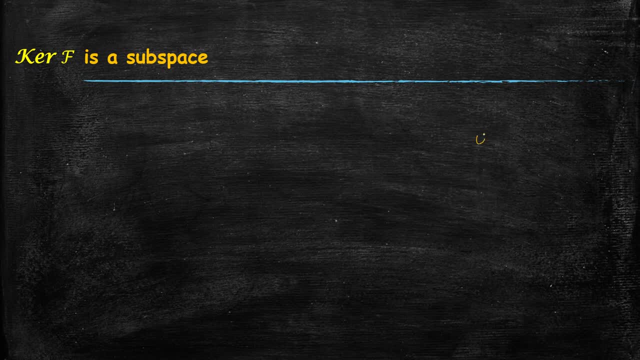 The dimension of image of f is called rank of f. Let moves to next theorem. Kernel of f is a subspace. Again, I will show that for every v1, v2 belonging to kernel of f, Alpha v1 plus beta v2 also belongs to kernel of f. 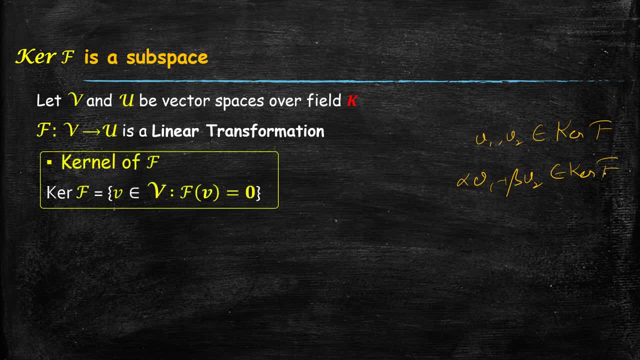 Let us start with the definition of kernel of f. Kernel of f are those elements of vector space v, Such that f equals to u. I assume v1, v2 be the elements of kernel of f. By definition of kernel of f, 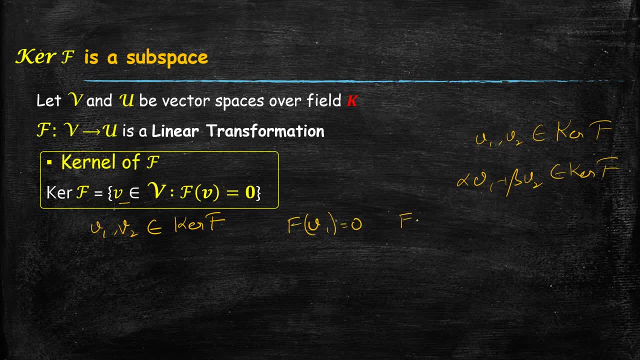 F of v1 is equal To 0.. F of v2 also equals to 0.. Now I have to show that alpha v1 plus beta v2 is also an element of kernel of f. For this I will prove that f of alpha v1 plus beta v2 is also equals to 0.. 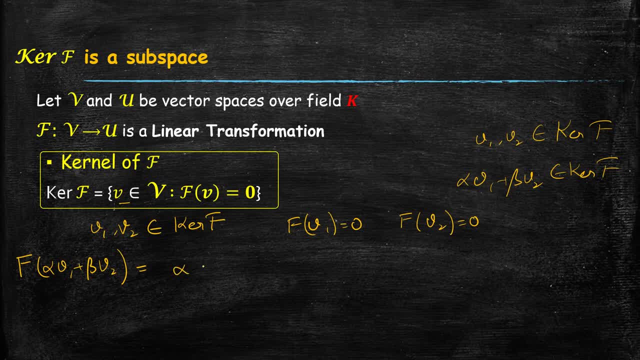 Now f is the linear transformation, So f of alpha v1 plus beta v2 equals to alpha of f v1 plus beta of f v2.. But f, v1, f, v2. Are equals to 0. So therefore we have equals to 0. 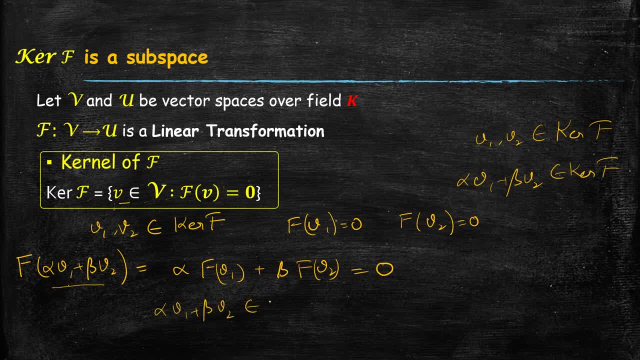 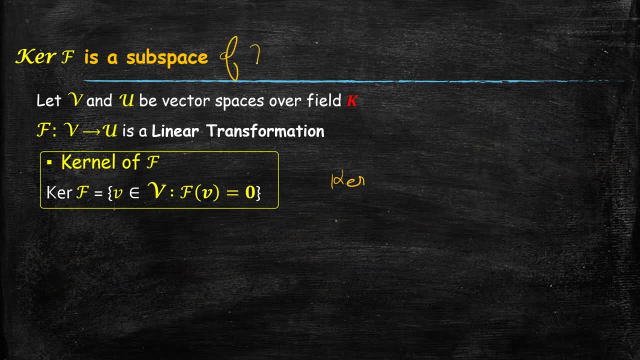 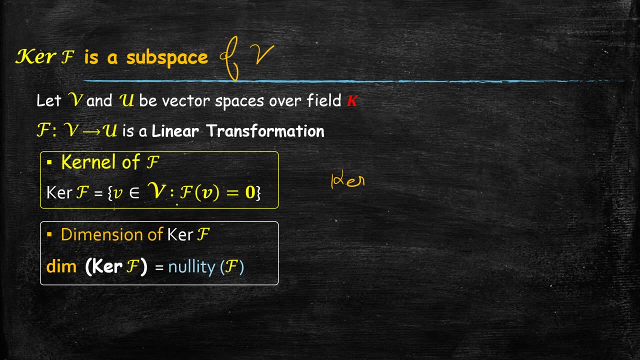 Alpha v1 plus beta v2 is also an element of kernel of f. So we can say that kernel of f is a subspace of vector space v. So kernel of f also has basis and there will be dimension of kernel of f. The dimension of kernel of f is called nullity of f. 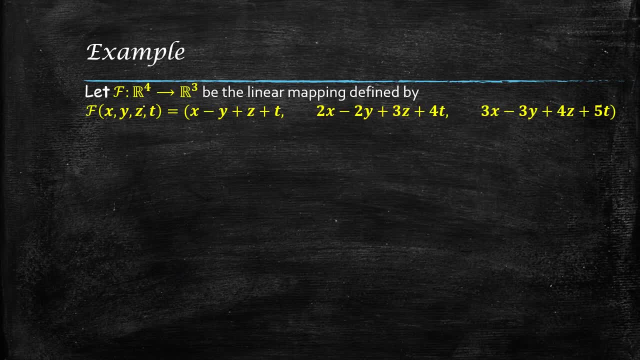 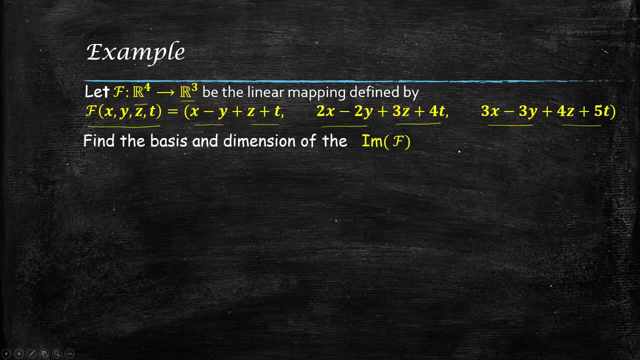 Let us explain it with the help of example. Let f be a Mapping from r4 to r3.. Now this mapping is a linear mapping, So our first question will be: find the basis and dimension of the image of f. Let us again consider our cat. 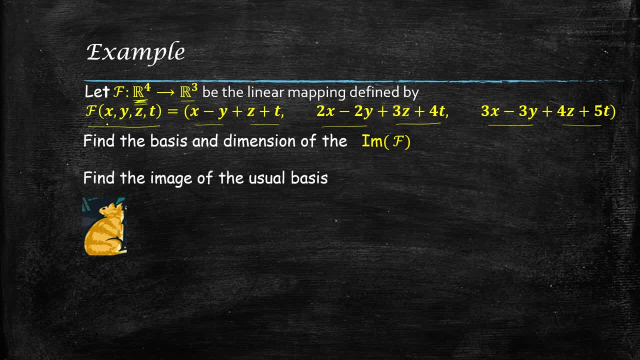 Whose image we have to find out. I will assume that cat be the usual basis. The usual basis here will be 1 0 0 0 0. 1 0 0 0 0. 1 0 0 0.. 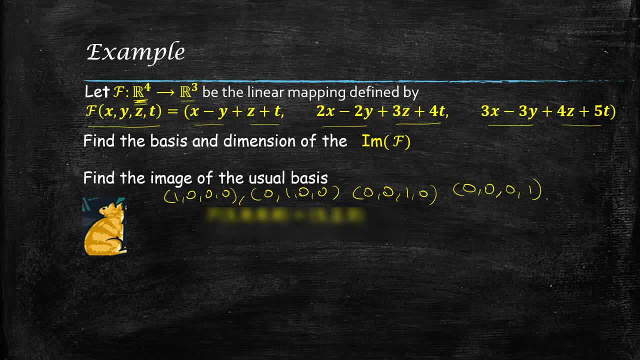 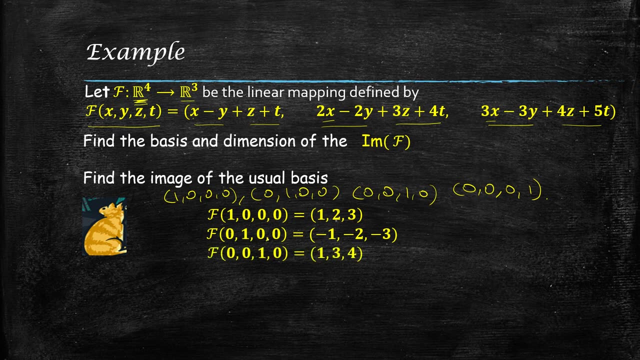 So this is our cat. Now we will find the tiger. f of 1 0 0- 0 is equals to 1, 2, 3. f of 0 1 0- 0 equals to minus 1 minus 2 minus 3. f of 0 0- 1- 0 equals to 1, 3, 4, and f of 0 0 0- 1 equals to 1 4, 5.. 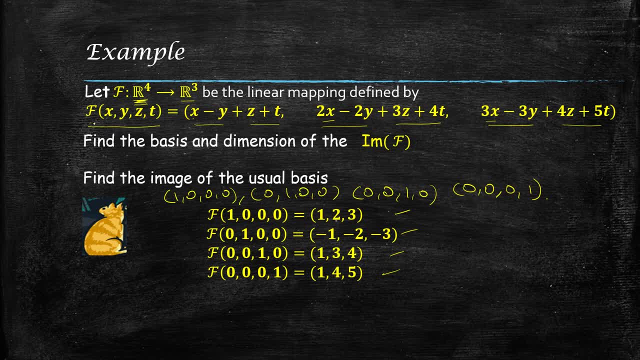 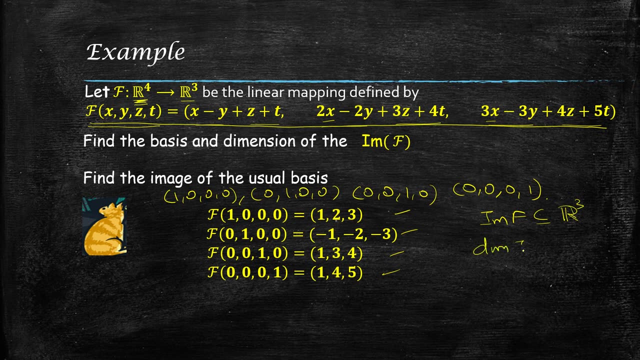 So we get these values from this linear transformation: f, x, y, z. But, as you know, that image of f is a subset of a vector space, r3, and the dimension of r3 is 3.. So dimension of image of f will always be less than or equals to 3.. 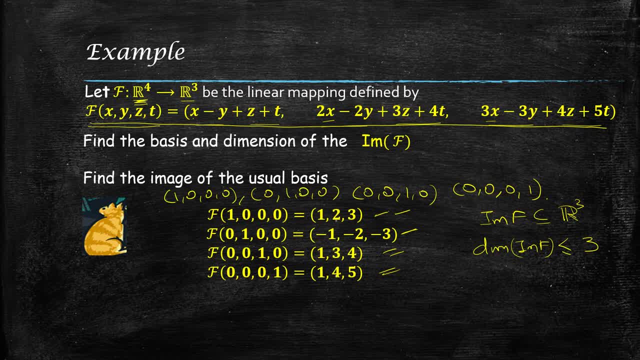 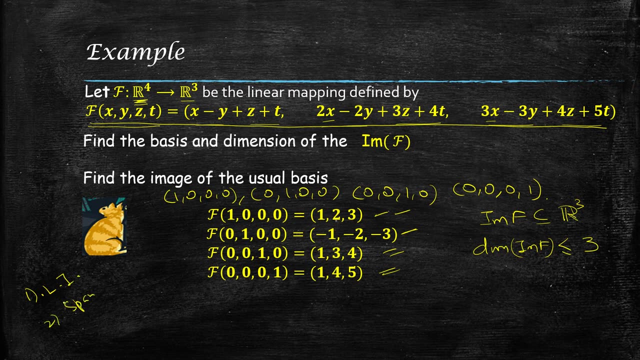 But here you have four vectors. These four vectors could not form the basis of the image of f Because these are not linearly independent. A set of vectors to be a basis, it must be linear independent. Second, It must span image of f. 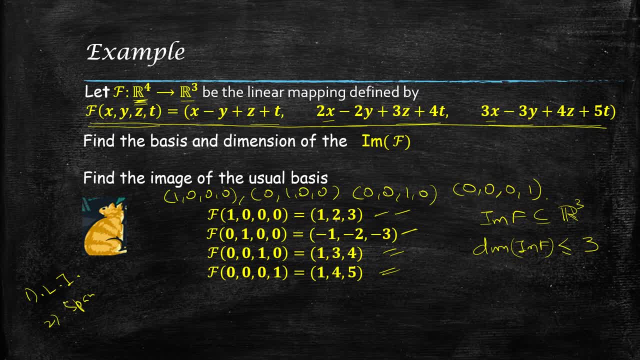 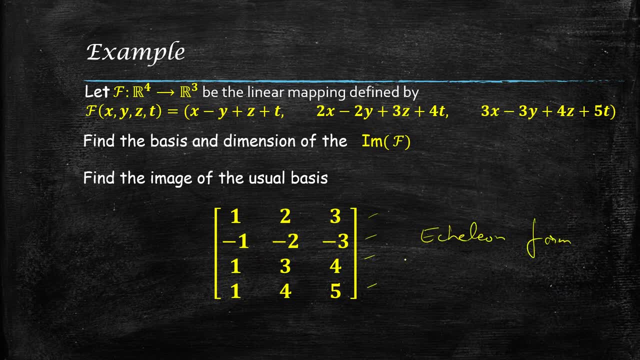 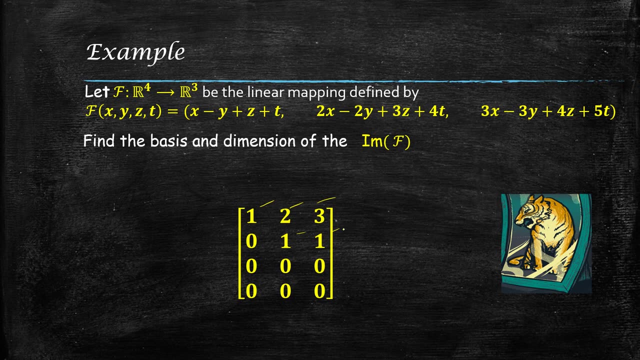 So, in order to find the basis of the image of f, we will write these set of vectors as a matrix and we will reduce this matrix to echelon form. We will operate on this matrix and this is our tiger: 1, 2, 3, 0, 1, 1.. 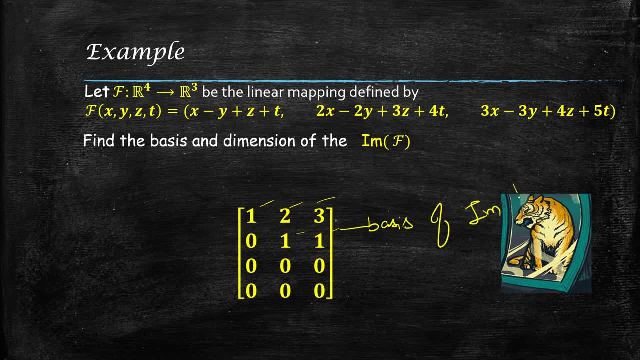 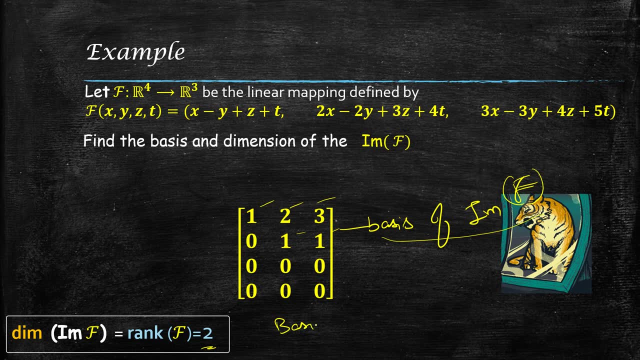 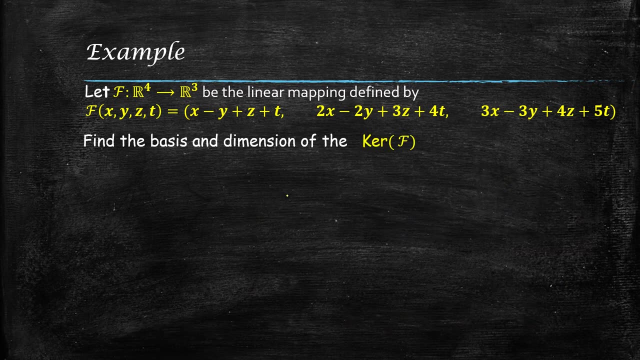 This is the basis of image of f, and dimension of image of f equals to 2, which is also called rank Basis. here is vector 1, 2, 3 and vector 0, 1, 1.. We will find the basis and dimension of the kernel of f. 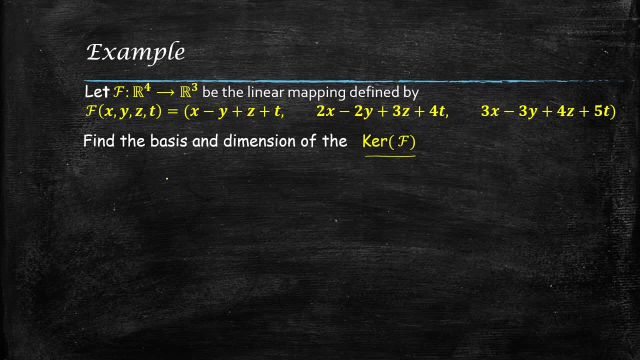 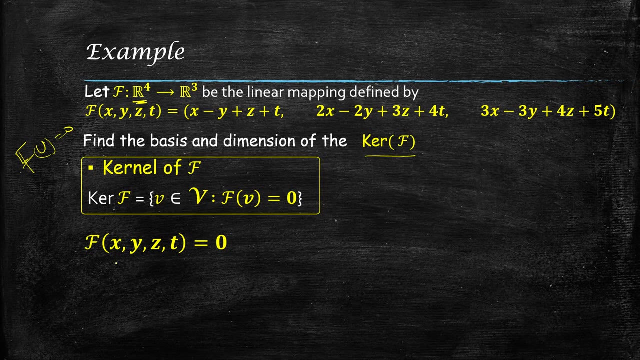 Now you know that kernel of f is defined as those elements of vector space v, such that f of v equals to 0.. So here let x y z. So here let x y z t be that element of r3.. Such that f of f, x y z t equals to 0. 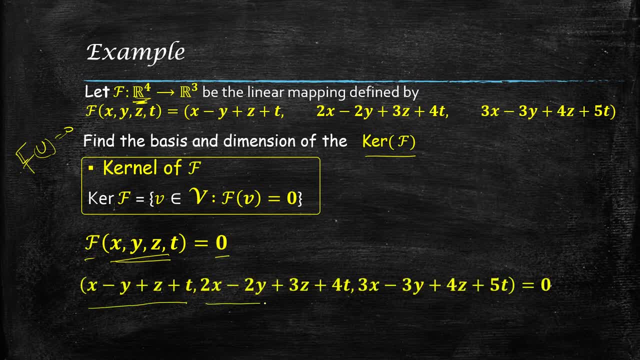 This means x minus y plus z plus t, 2x minus 2y plus 3z plus 4t. 3x minus 3y plus 4z plus 4t equals to 0.. We will get here the homogeneous system of linear equations. 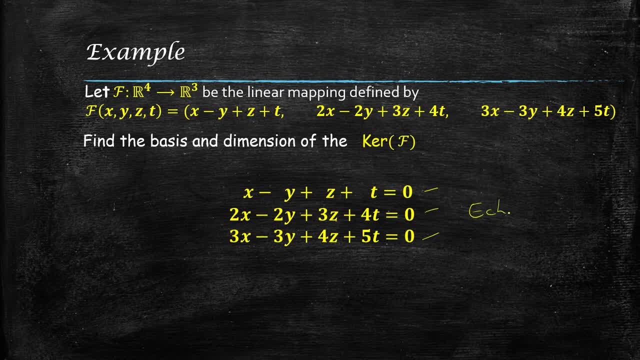 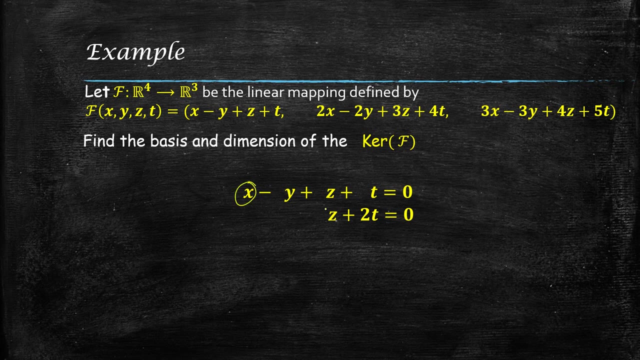 Three linear equations. We will reduce this system to echelon form in order to find out the basis. Now, number of equations are less Than number of unknowns, So this system has non-zero solution, Reducing it to echelon form. There are two leading unknowns, x and z, and two free variables, y and t. 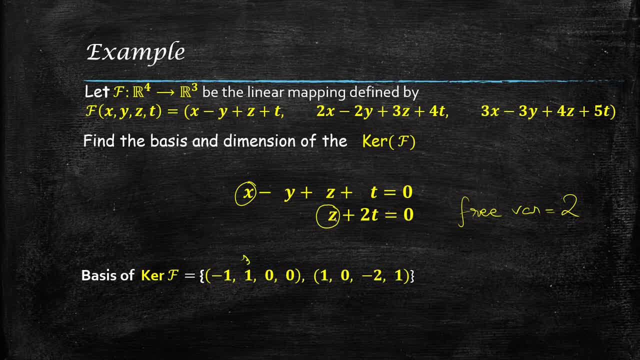 In order to find the basis, I will put y equals to 1, t equals to 0.. So our first vector will be minus 1, 1, 0, 0.. Again, put y equals to 0 and t equals to 1.. We will get our second non-zero solution. 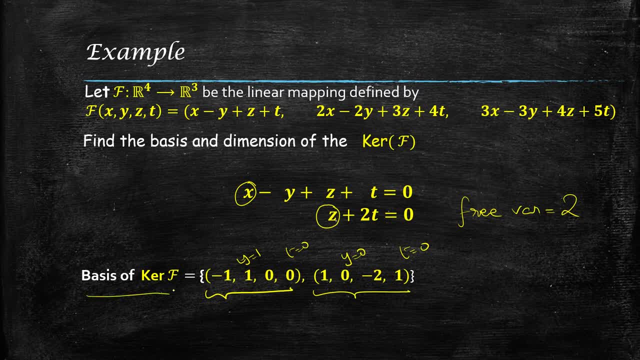 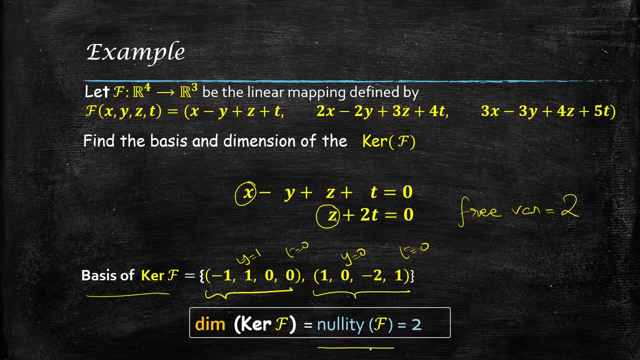 1, 0 minus. So this is the basis of kernel of f And the dimension of kernel of f is equals to also called nullity of f. So I think it is clear that if you have been given a linear transformation, Then you can easily find the basis and dimension of image of n and kernel of f.